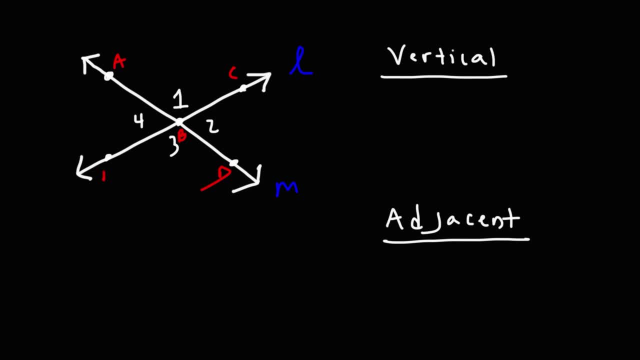 C, D and E. So angles 1 and 3 are vertical angles. They're across from each other and vertical angles are congruent. They have the same angle measure. You can also call angle 1 as angle ABC. Angle 3 is EBD or you can say DBE. Notice that these two angles, they share a common vertex. 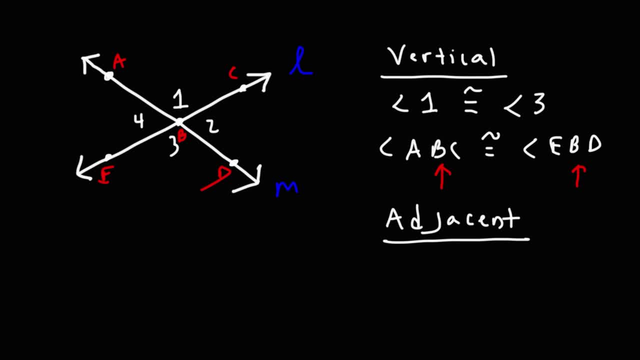 which is located at point B. So vertical angles are angles that share a common vertex, They're congruent and they exist across from each other. So 1 and 3 are vertical angles. also, 2 and 3 are vertical angles And 4 are vertical angles, Adjacent angles. they're angles that share the 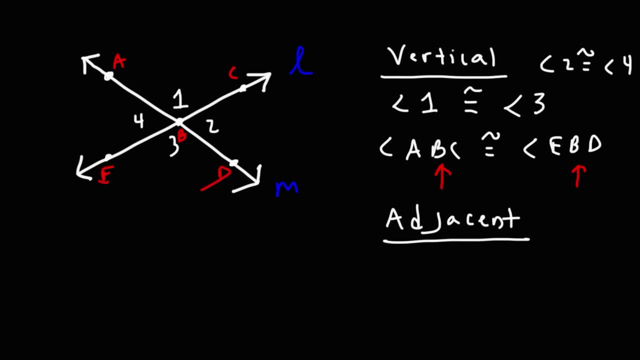 same vertex, but they also share one ray or one side. So angles 1 and 2 are adjacent angles. They're adjacent to each other, They're right next to each other. So let's write that here. So 1 and 2 are adjacent. So that would be angle ABC and angle CBD. 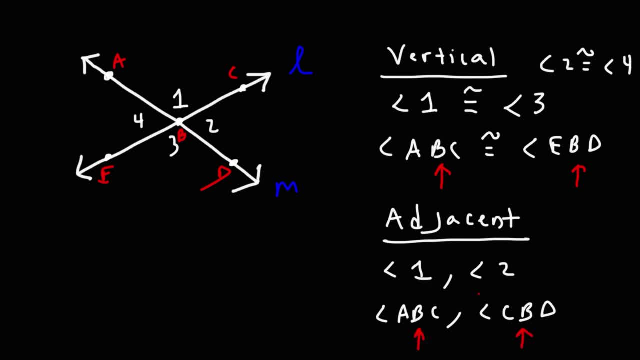 As you can see, they share a common vertex, B, But now I'm going to color it. So that's angle 1, ABC and also angle 2, CBD. The common ray or the common side of the vertex that they share is ray BC. So those are adjacent angles. They're angles that are right next to each. 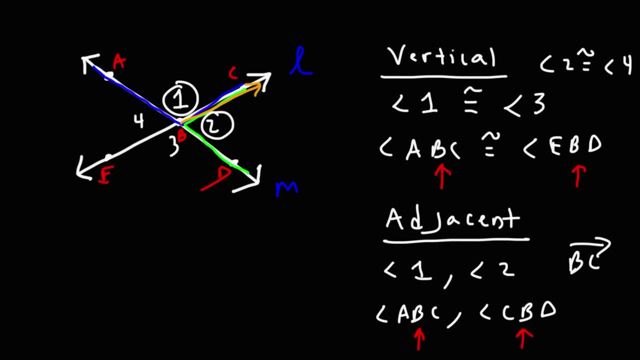 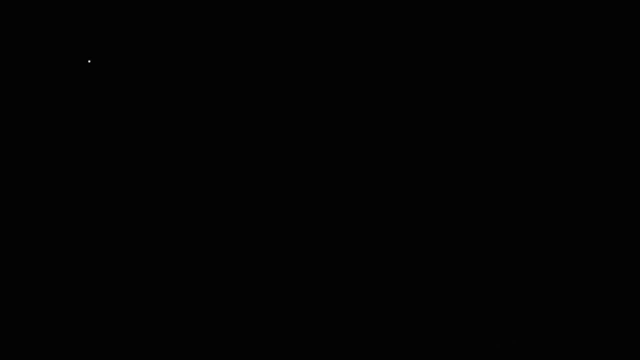 other. They share a common vertex and they share a ray. Now there are different types of adjacent angles. When you have a right angle and you add a ray to it, you're going to have a common vertex. You can create two adjacent angles, In this case angle 1 and angle 2.. Now these two angles, even 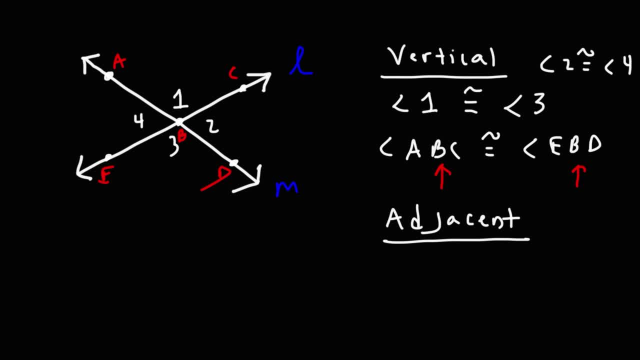 vertex, but they also share one ray or one side. So angles one and two are adjacent angles. They're adjacent to each other, they're right next to each other. So let's write that here. So one and two are adjacent, so that would be angle ABC. 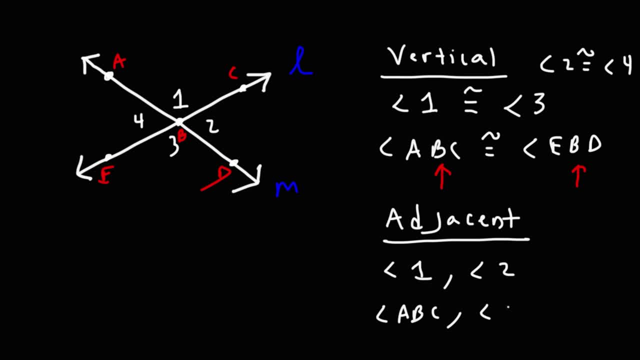 and angle CBD. As you can see, they share a common vertex B, But now I'm going to color it. So that's angle one ABC and also angle two CBD. The common ray or the common side that they share is ray BC. So those are. 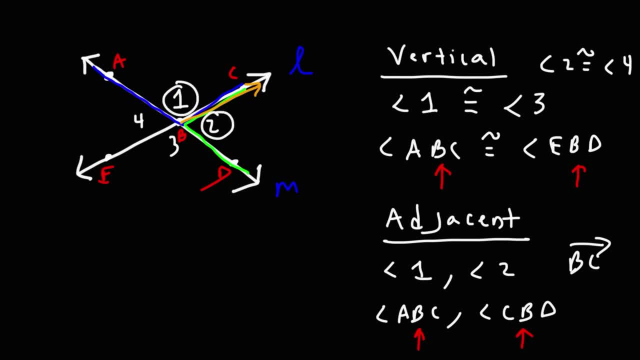 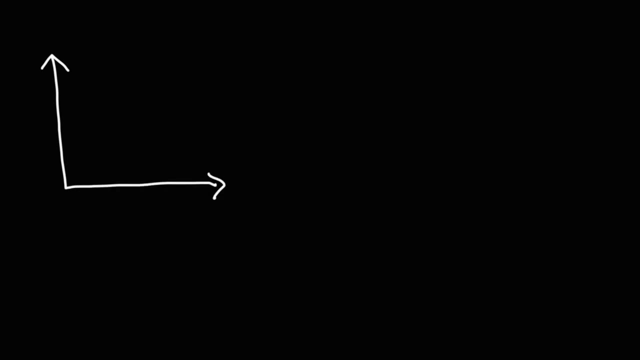 adjacent angles. They're angles that are right next to each other. they share a common vertex and they share a ray. Now there are different types of adjacent angles. When you have a right angle and you add a ray to it, you can create two adjacent angles, In this case, angle. 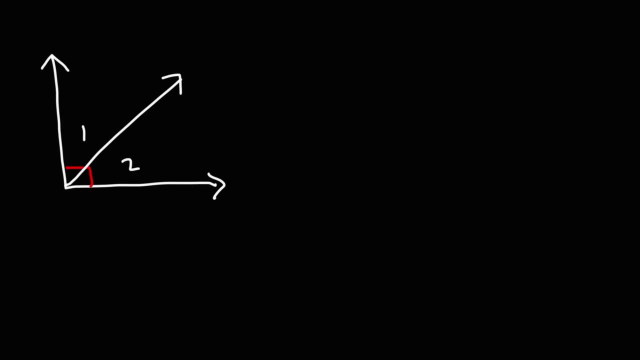 one and angle two. Now these two angles, even though they're adjacent, there's another special term that describes the relationship. Those angles are complementary, Complementary angles. they add up to 90 degrees. Now two adjacent angles can also form a linear pair. When that happens, the angles 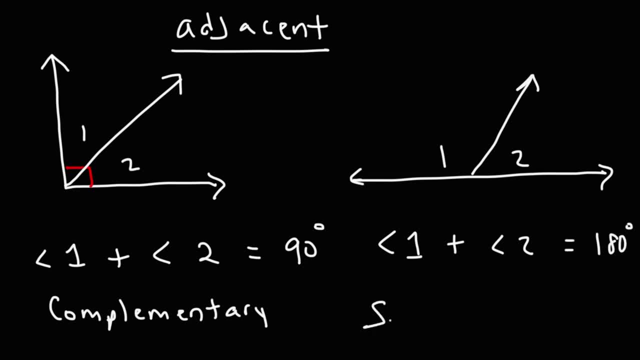 add up to 180 degrees. In this case we would say that they're supplementary angles, even though they're still adjacent to each other. So now you know the difference between vertical angles and adjacent angles, And you also know the difference between complementary angles. 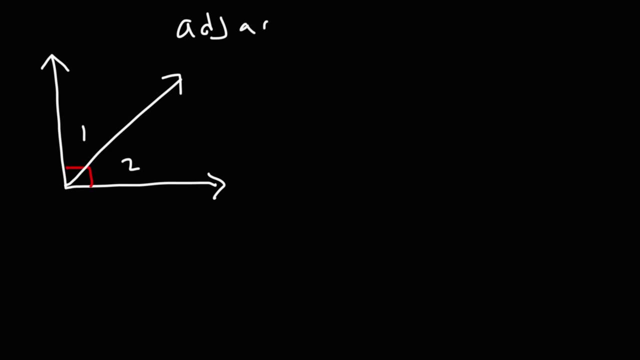 though they're adjacent, there's another special term that describes the relationship. Those angles are complementary, Complementary angles. they add up to 90 degrees. Now two adjacent angles can also form a linear pair. When that happens, the angles add up. 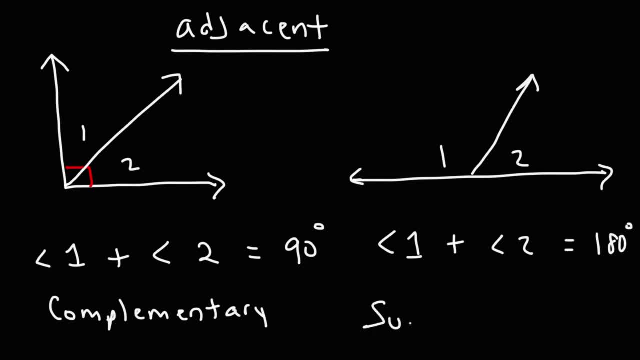 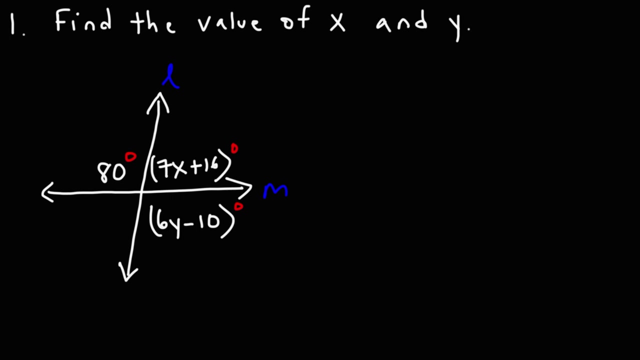 to 180 degrees. In this case, we would say that they're supplementary angles, even though they're still adjacent to each other. So now you know the difference between vertical angles and adjacent angles. Subtitles by the Amaraorg community. Now let's try this problem. So we have two lines, line L and M, and we have the angles. 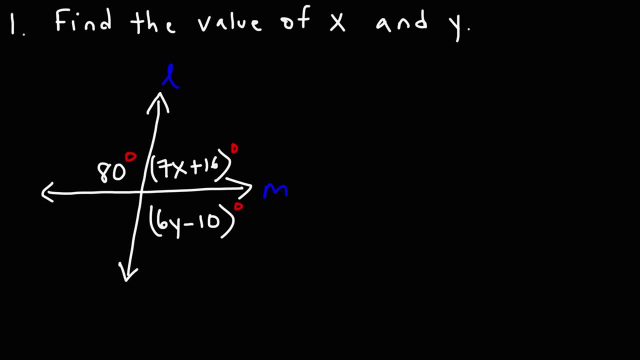 some, in terms of x and y, Find the value of x and y in this problem. Now, let's call this angle 1.. I'm just going to put a 1 here. We'll call this angle 2 and angle 3, just to keep things simple. 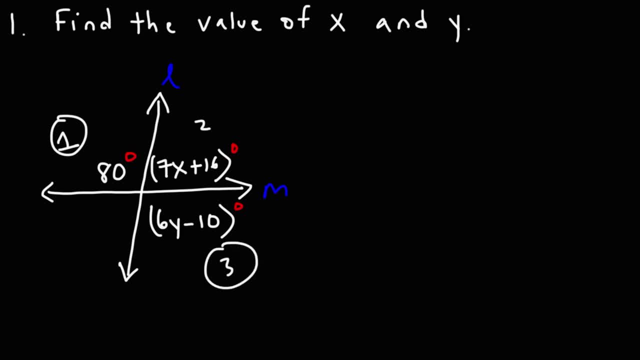 Angles 1 and 3, we know that they're vertical angles- They're across from each other, So we can set them equal to each other. So angle 1 is equal to angle 3.. I wrote 2 for some reason. 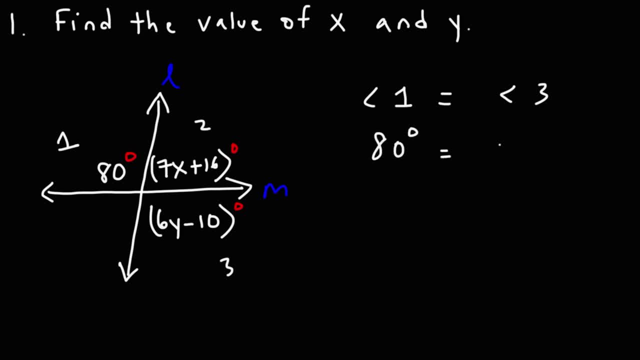 Angle 1 has a measure of 80 degrees, And angle 3 is equal to angle 3.. And angle 3 is equal to angle 3. And angle 3 is 6y minus 10.. So now we just have to solve for y. 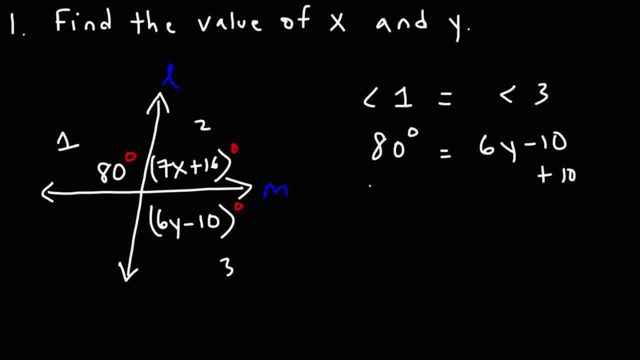 Let's add 10 to both sides, So we're going to have: 90 is equal to 6y, And then we could divide both sides by 6.. 90 divided by 6.. Well, if you want to do this without a calculator, 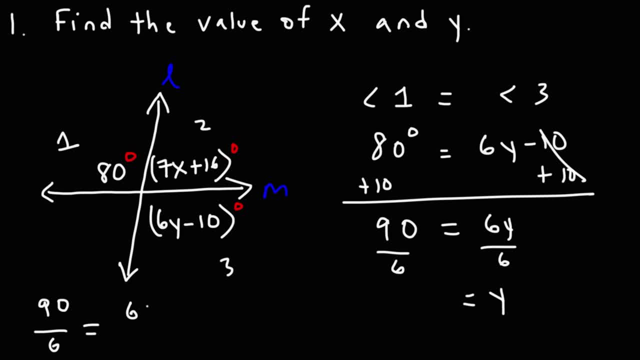 it helps if you break up 90 into 60 and 30.. 60 divided by 6, that's 10.. 30 divided by 6 is 5,, so you get 15.. So that's the value of y. 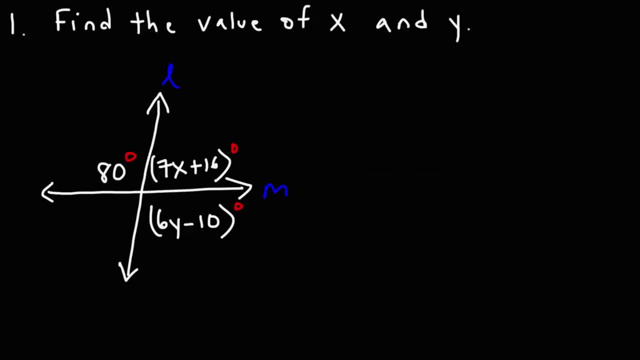 and supplementary angles. Now let's try this problem. So we have two lines, line L and M, and we have the angles, some in terms of x and y. Find the value of x and y in this problem. Now let's call this angle 1.. I'm just going to put a 1 here. We'll call this. 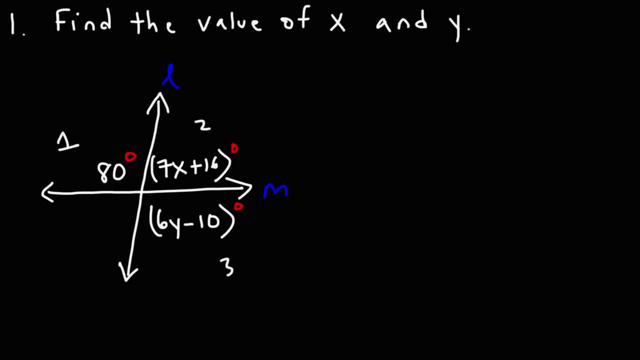 angle 2 and angle 3, just to keep things simple, Angles 1 and 3, we know that they're vertical angles, They're across from each other, So we can set them equal to each other. So angle 1 is equal to angle 3.. 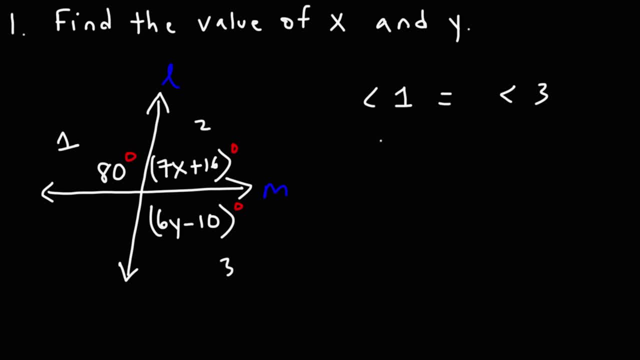 I wrote 2. for some reason, Angle 1 has a measure of 80 degrees and angle 3 is 6y minus 10.. So now we just have to solve for y. Let's add 10 to both sides, So we're going to have 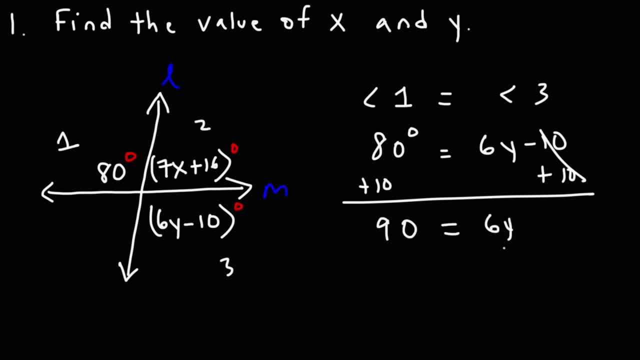 90 is equal to 6y, and then we could divide both sides by 6.. And Fre quantum acceleration is 90 divided by 6,. well, if you want to do this without a calculator, it helps if you break 90 up into 60 and 30. That's 10.. 30 divided by 6. 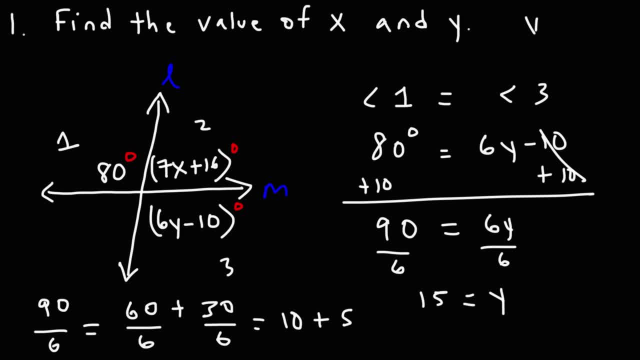 is 5, so you get 15.. So that's the value of y, y, which equals 15.. $5.00$5.00$3.00$4.00$5.00$5.00$. Well, we could say technically 15 degrees. 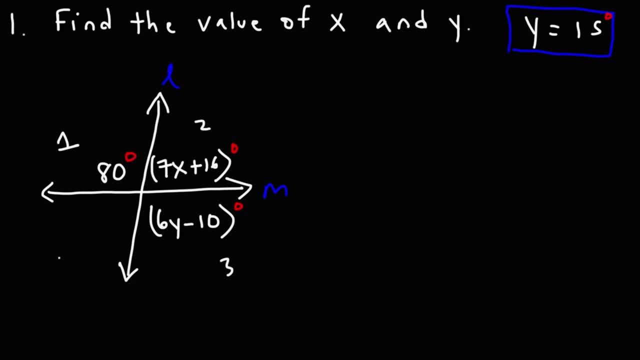 Now, what about X? Angles 1 and 2, they are adjacent. These angles are right next to each other. Now, M is a line. Lines have an angle of 180.. Lines are straight. So this right here is 180, which means angles 1 and 2, they're not only adjacent but they're supplementary. 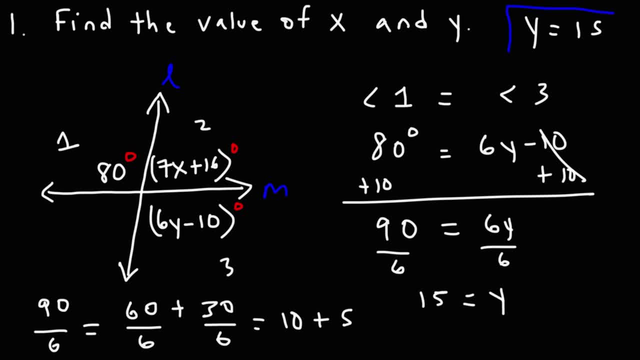 y is equal to 15.. Well, we could say, technically, 15 degrees. Now what about x? Angles 1 and 2, they are adjacent. These angles are right next to each other. Now m is a line. 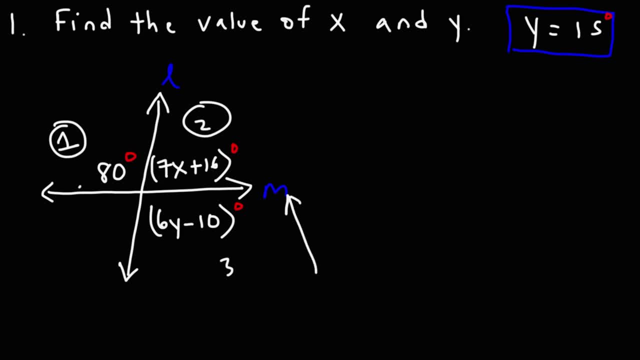 Lines have an angle of 180.. Lines are straight, So this right here is 180, which means angles 1 and 2, they're not only adjacent, but they're supplementary, So we could say that 80 is equal to 180. 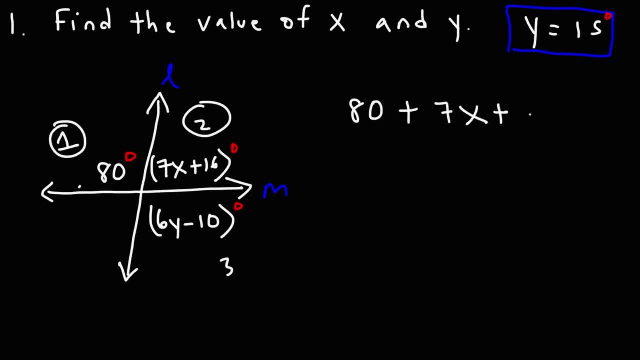 80 plus 7x plus 16, that's going to add up to 180.. Now let's begin by subtracting both sides by 80.. So we get 7x plus 16 is equal to 180. minus 80 is 100. 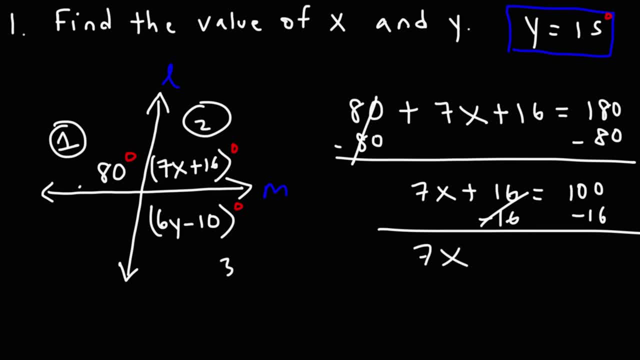 And then we could subtract this by 16. 100 minus 16 is 84. And then divided by 60. And then divided by 7. So 84 divided by 7. 70 goes into, I mean 7 goes into 70. nicely. 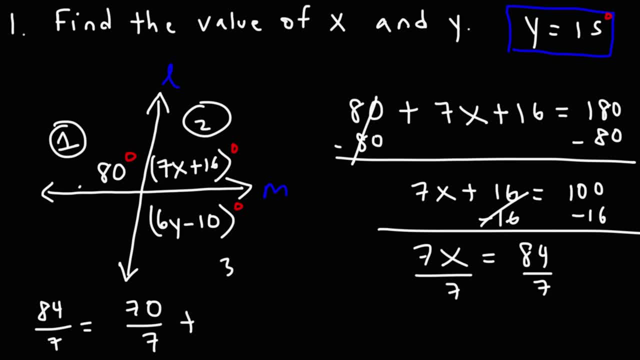 And 84 minus 70 is 14.. So 70 divided by 7 is 10.. 14 divided by 7 is 2.. So x is going to be 12.. So now we know the value Of x and y. 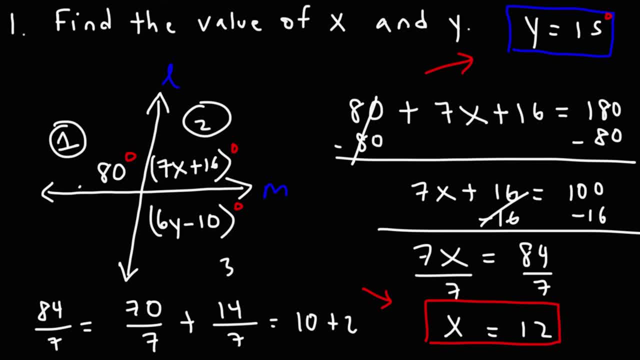 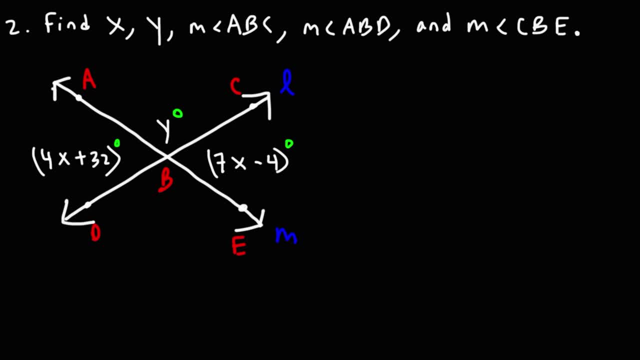 x is 12,, y is 15.. Let's try this problem. So, given the diagram shown below, Find the values of x, y, the angle measure of ABC, ABD and CBE, And we're given lines L and M. 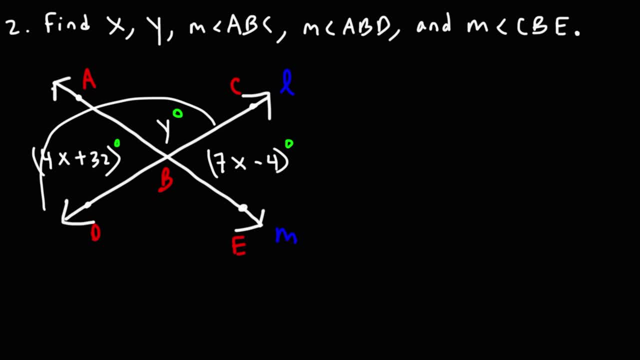 So we know these two angles. They're supplementary and adjacent, And the same is true with those two angles. The problem, though, is we have two different variables, So we don't want to touch that yet. What we could do is set these two vertical angles equal to each other. 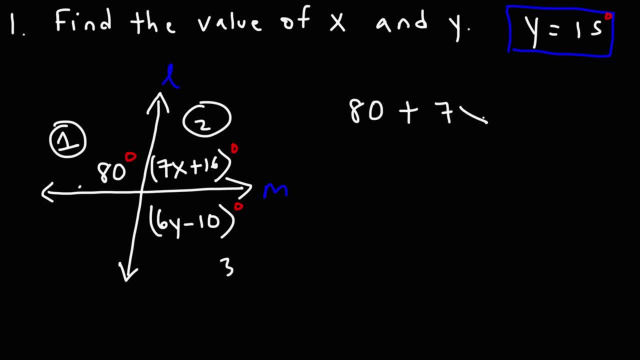 So we could say that 80 plus 7X plus 16, that's going to add up to 180.. Now let's begin by subtracting both sides by 80.. So we get: 7X plus 16 is equal to 180. minus 80 is 100. 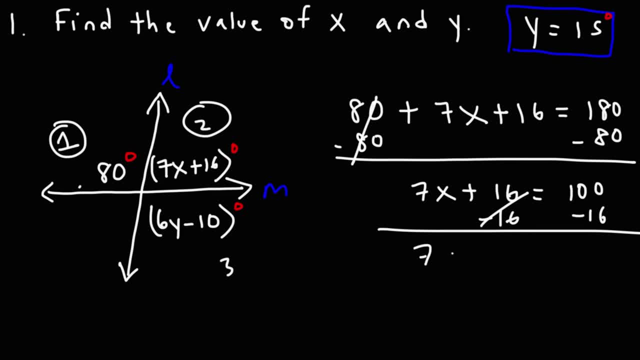 And then we could subtract this by 16. 100 minus 16 is 84. And then divide it by 7. So 84 divided by 7. 70 goes into, I mean 7 goes into 70. nicely. 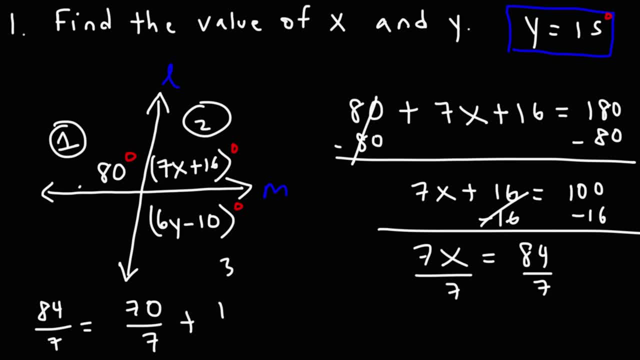 And 84 minus 70 is 14.. So 70 divided by 7 is 10.. 14 divided by 7 is 2.. So X is going to be 12.. So now we know the value of X and Y. 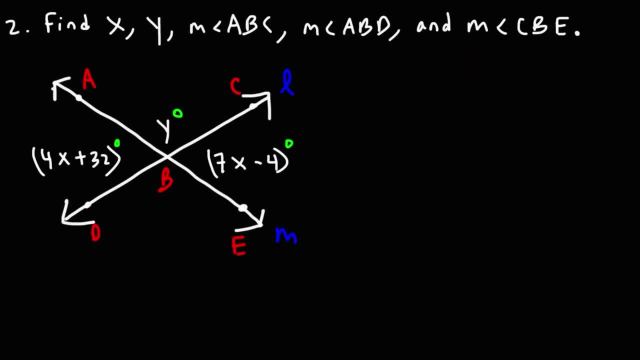 X is 12,, Y is 15.. Let's try this problem. So, given the diagram shown below, find the values of X, Y, the angle measure of ABC, ABD and CBE, And we're given lines L and M. 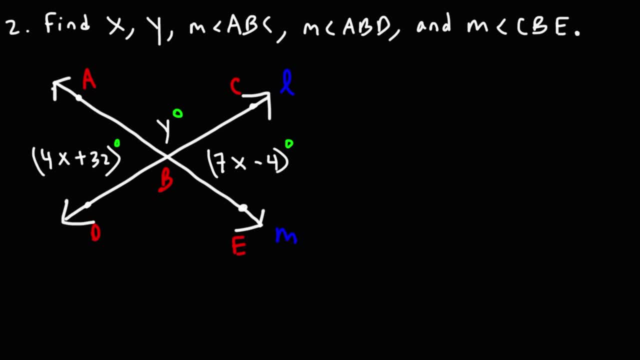 So we know these two angles. they're supplementary and adjacent, And the same is true with those two angles. The problem, though, is we have two different variables, So we don't want to touch that yet. What we could do is set these two vertical angles equal to each other. 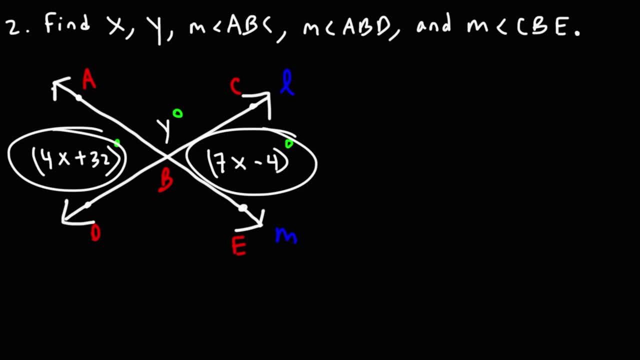 And since we have only one variable, X, we could find the value of that variable. So angle ABD is congruent, or we could just say it's equal to angle CBE, Because they're vertical angles. Now, angle ABD, which is this part here, that's 4X plus 32.. 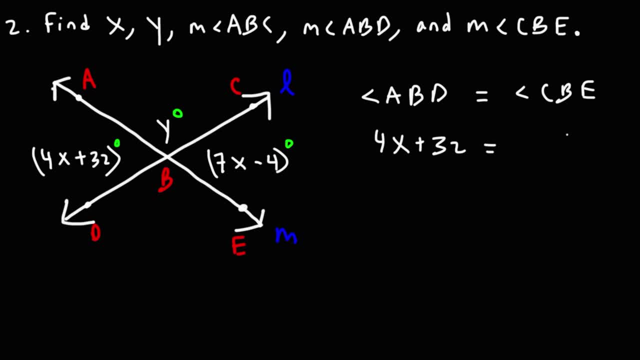 And CBE is 4X plus 32.. 7X minus 4.. Now let's solve for X. So I'm going to add 4 to both sides And I'm going to subtract by 4X from both sides. 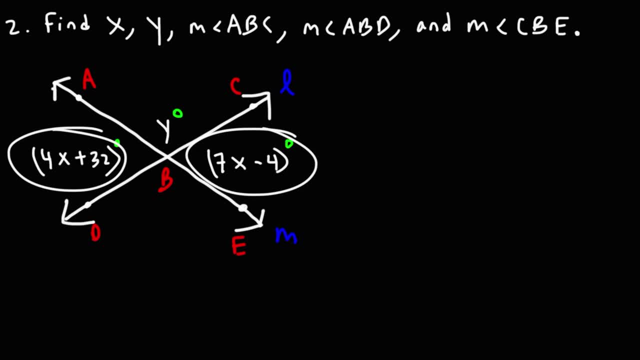 And since we have only one variable, x, We could find the value of that variable. So angle ABD is congruent, Or we could just say it's equal to angle CBE, Because they're vertical angles. Now, angle ABD, which is this part here. 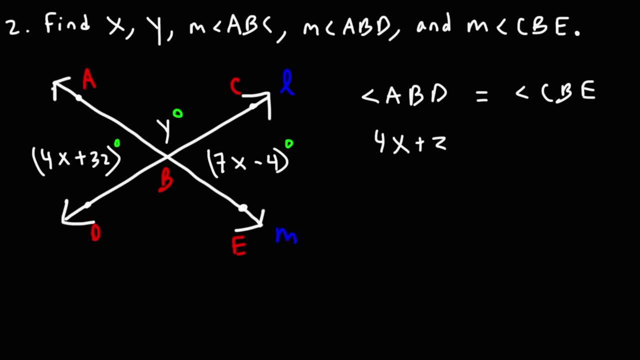 That's 4x plus 32. And CBE is 7x minus 4.. Now let's solve for x. So I'm going to add 4 to both sides And I'm going to subtract by 4x from both sides. 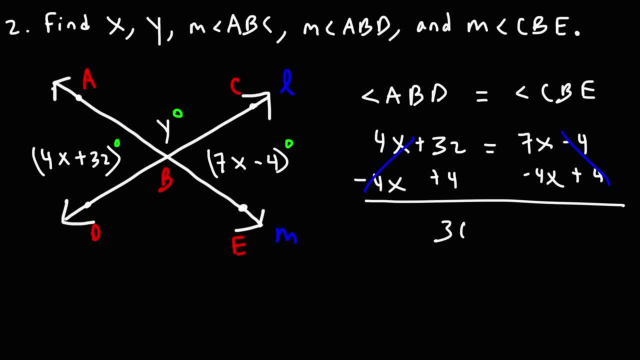 So we can cancel that. 32 plus 4 is 36.. 7 minus 4 is 3.. So we get: 3x is equal to 36.. Now let's divide both sides by 3.. 36 divided by 3 is 12.. 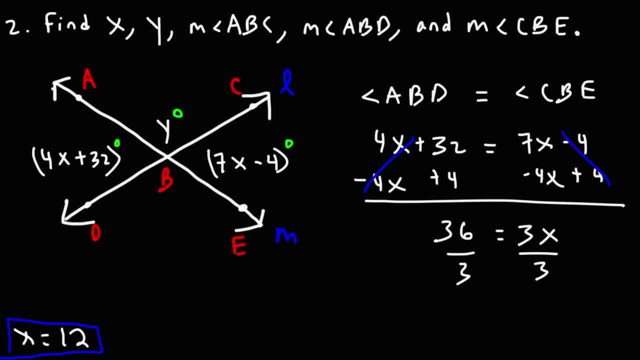 So we now know the value of x. So now that we have that, We could find the angle measure of angle ABD. So angle ABD, That's 4x plus 32.. Replace an x with 12.. Replace an x with 12.. 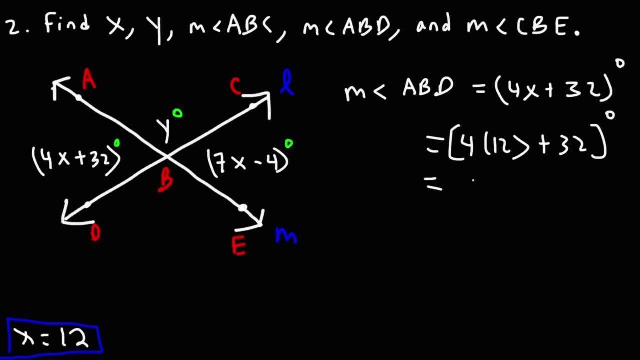 We get 4x12, which is 48.. 48 plus 32, that's going to be 80. So the measure of angle ABD is 80.. Now ABD and CBE, they're vertical angles, So they have the same measure. 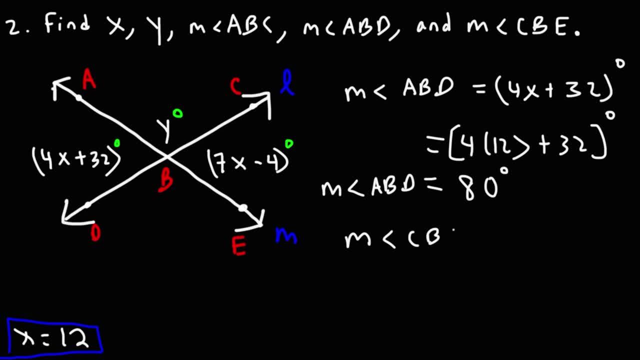 Therefore angle CBE is also 80.. So this is 80 degrees, This is 80 degrees. We can easily find y. So these two angles, they form a linear pair, They're supplementary. So y plus 80 is 100.